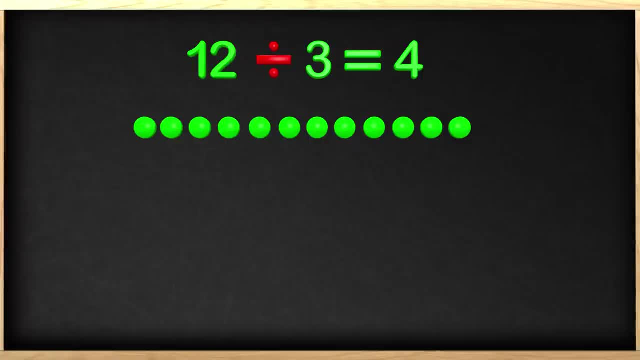 notice that the twelve is at the beginning. In a division problem you start with the total number of dots. The problem is telling us that we will take twelve dots and divide them equally among three groups. We will put a dot in each group until all dots are gone. 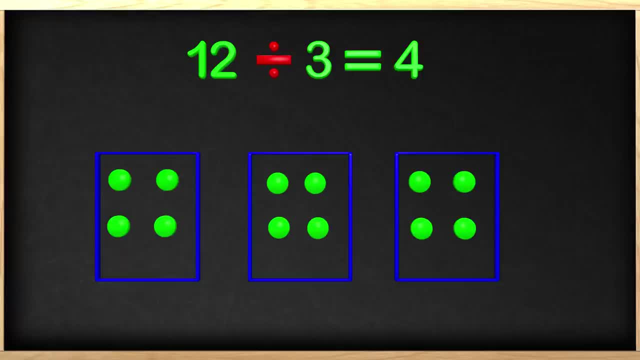 Can you tell me how many dots are in each group? There are four dots in each group. just like the answer: Awesome. In both the multiplication and division problems, the smaller numbers tell us how many groups we have and how many items go in each group. The biggest number in each problem is the. 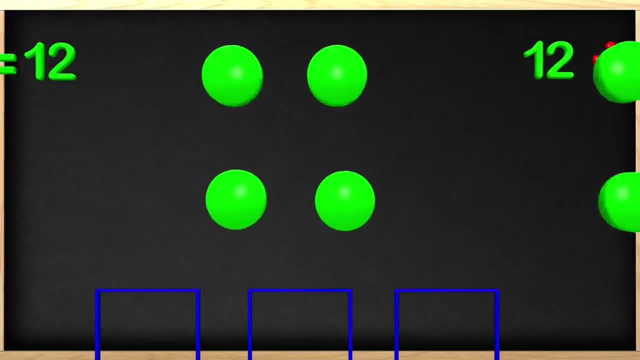 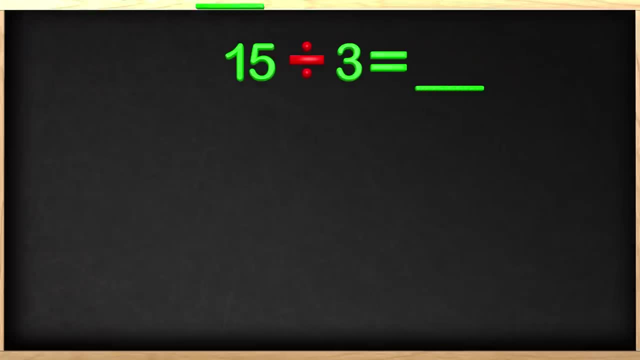 total amount of items or dots in our case. Here are two more problems, but they don't give us the answer. Let's start with the division problem and see if using multiplication can help us. Fifteen divided by three equals blank. Fifteen is the large number or total of dots We are. 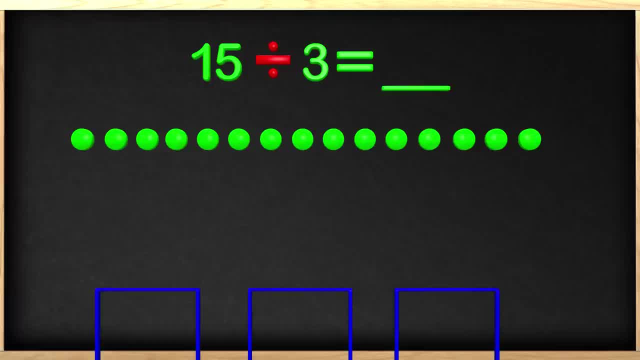 dividing the fifteen dots equally among three groups. We start by using our three groups and share the dots equally. To do this, we will put one dot in each group until they are gone. How many dots are in each group? The answer is five. Great job. So fifteen divided by three is five. If we pay attention, we can. 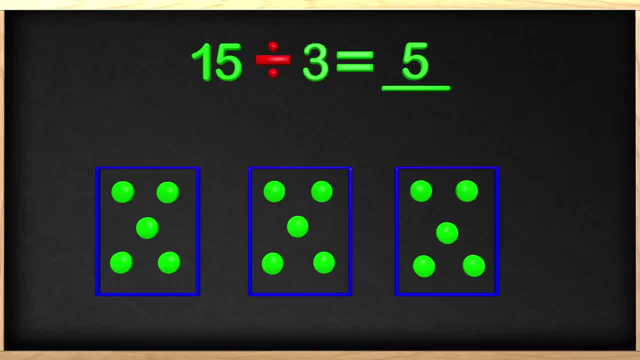 see that five multiplied by three in the problem gives us fifteen. Wait a minute. We just answered the multiplication problem on the left. Five times three equals fifteen. It's really important to remember that in division you are finding what two numbers multiply by three, The answer. 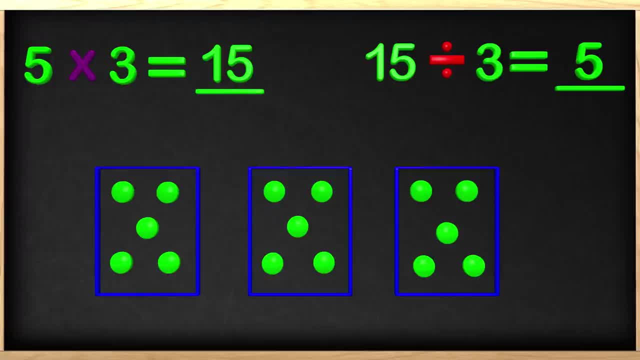 is five. Five multiplied together equals the largest number. The two smaller numbers in this division problem multiplied together gives us the largest number, which is fifteen. This is amazing stuff, and now it is time to go play some tag. This time I am going. 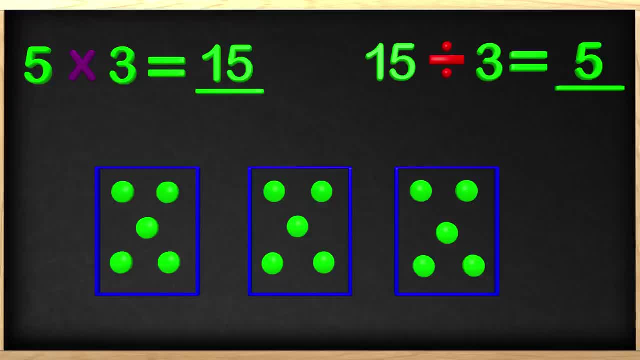 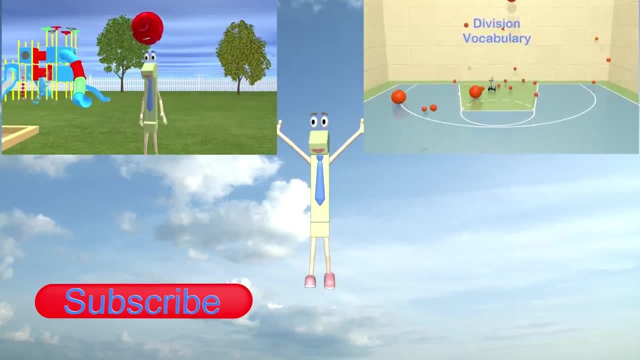 to be ready now that I understand a little bit more of division and multiplication. See you next time, Goodbye. Okay, guys, you have a few options here. You can click the video on my right or on my left to watch more awesome stuff.